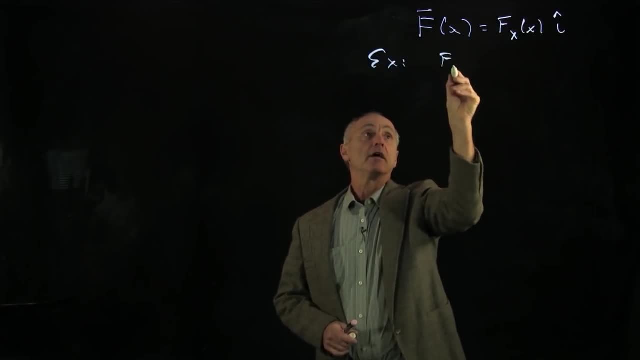 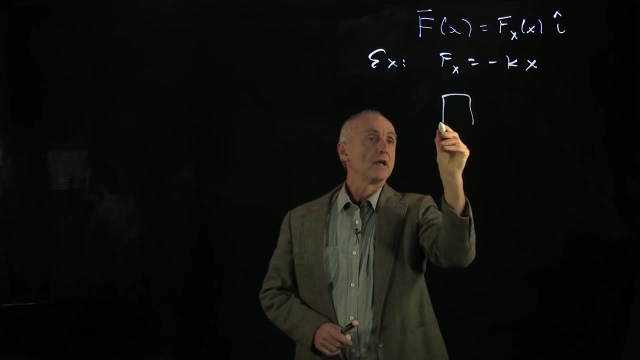 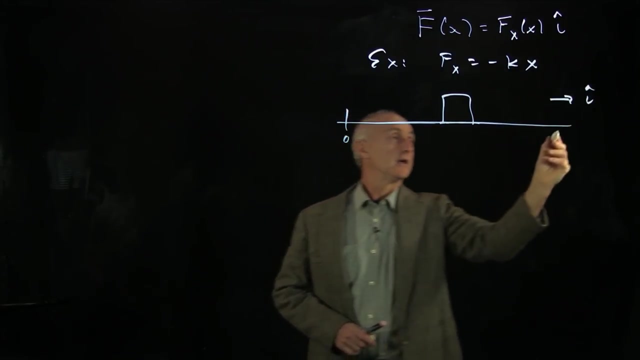 And one of the simplest examples of a force like this is what we call the spring force. Now, when we apply this force to our object- and let's look at an object- i i-hat direction will have an origin, And this is our plus x coordinate system. Now, when we apply a 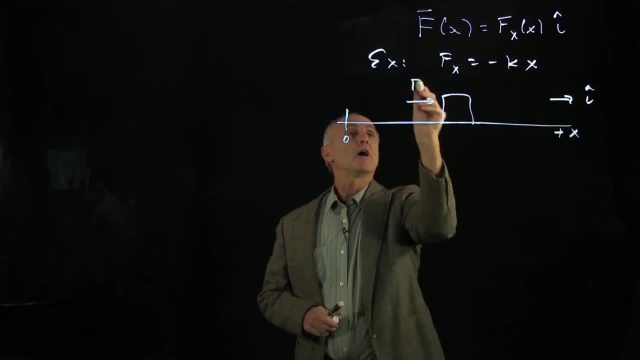 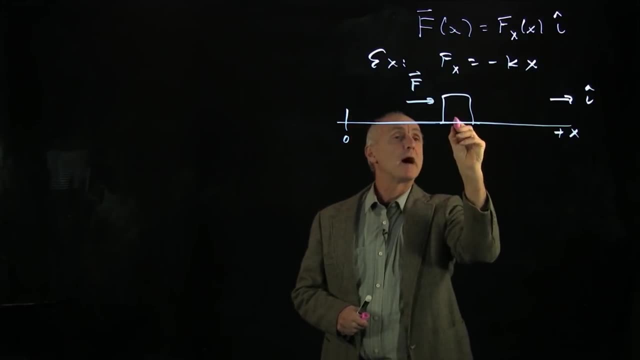 force. what we want to look at is because the force is a function of position. then we want to look at the displacement over a small amount. So let's call this the point xj out here. let's refer to this as xj plus 1.. 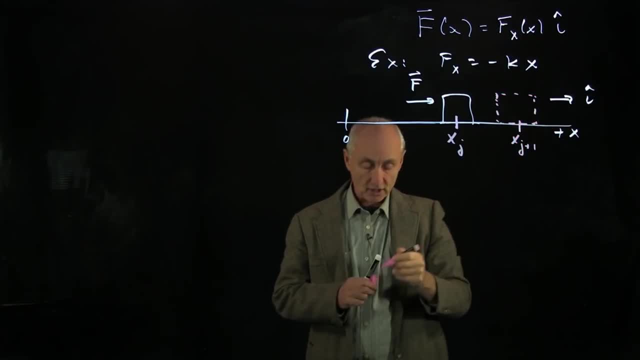 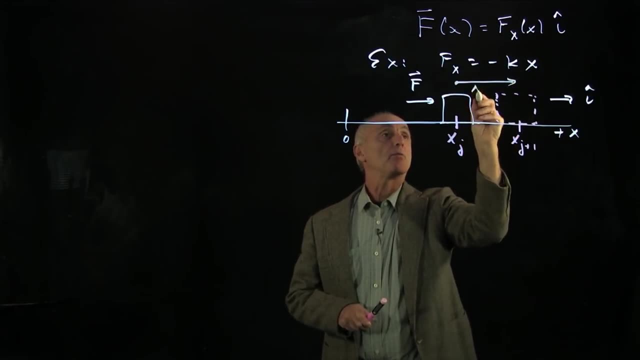 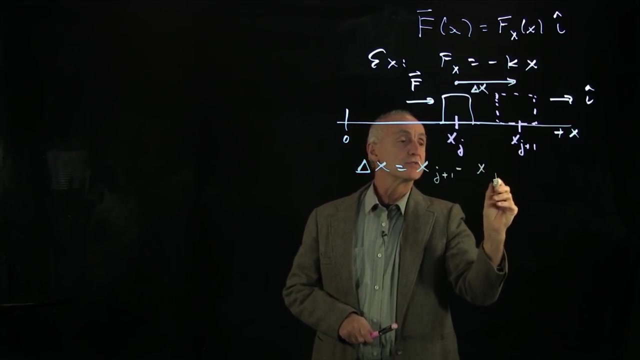 And what we've done is we're going to ask how much work is done when the force is displaced from here to there, And that's what we'll call delta x. So now our displacement is a small displacement: x of j plus 1 minus x of j. 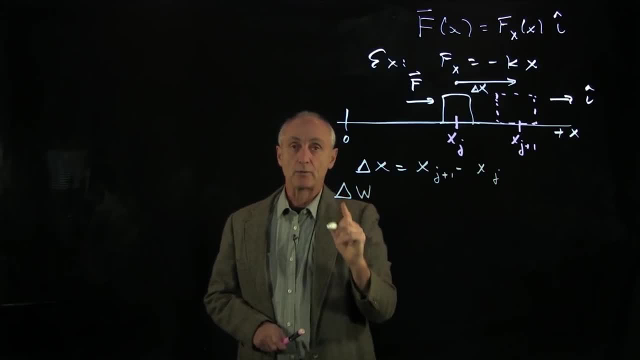 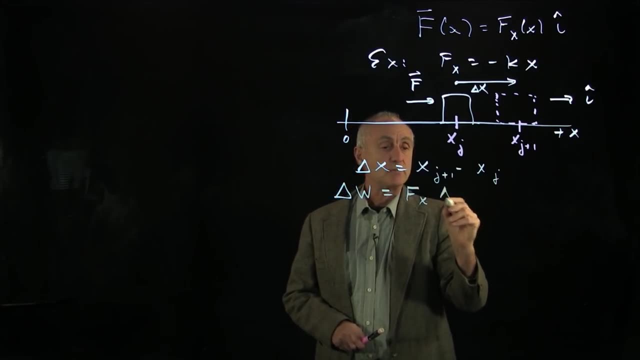 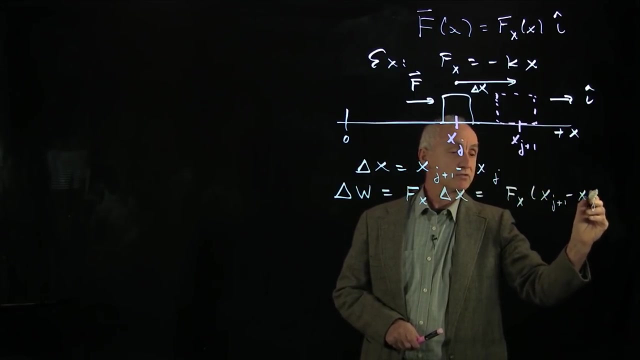 And our work for this small displacement- and that's why we'll indicate it with a delta- is equal to the force which is a function of x times this displacement. And so now we get f of x times x of j, plus 1 minus x of j. 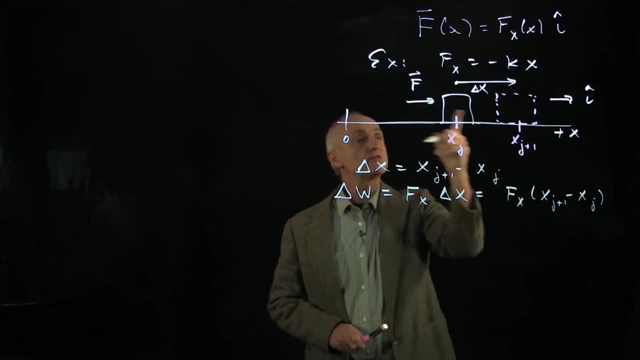 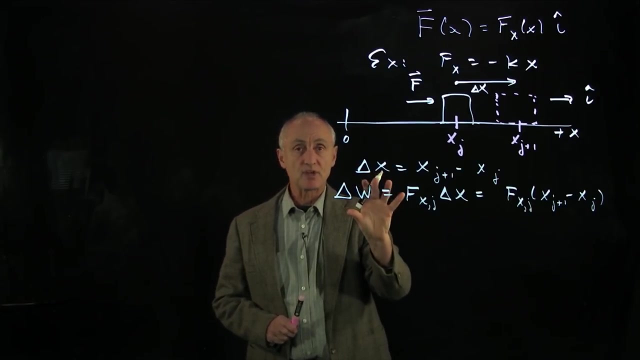 And what we have to indicate here is because the force is varying. we're looking at just this displacement here. Let's refer to this force as in the jth part. Now, the total work, It's just the sum of all these scalar quantities. 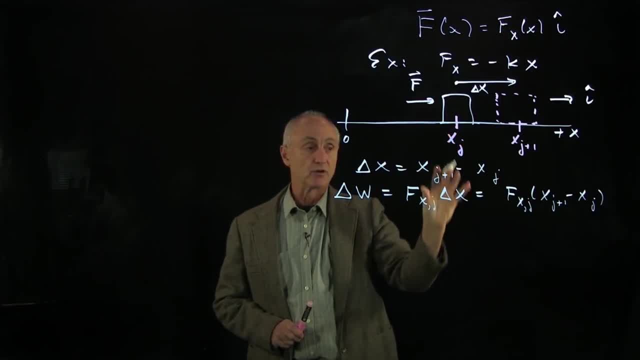 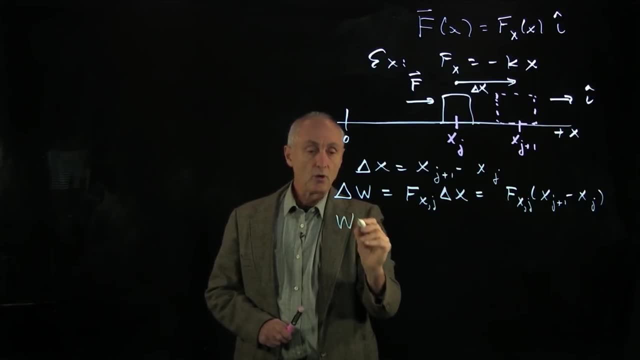 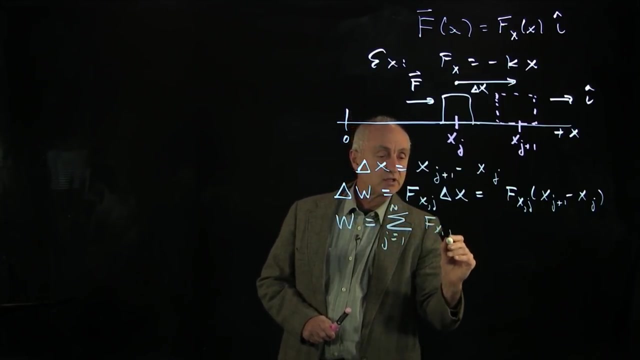 Remember, although force is a vector and displacement is a vector, the product of these two quantities is a scalar. And so if we want the total work, we have to sum from: j goes from 1 to n of this quantity f of j dot, and I'll put a little j there to indicate that. 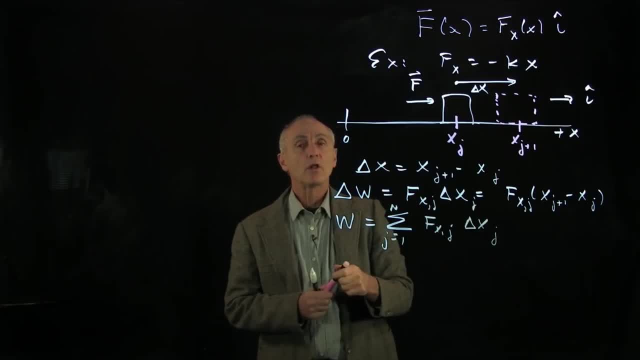 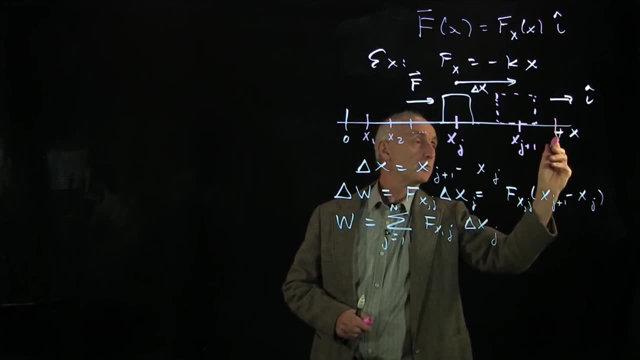 delta xj. Now, what does this sum mean? Well, imagine that we're making a series of, let's say, displacements all the way out to a final position, x final, and we have divided this interval into n pieces. 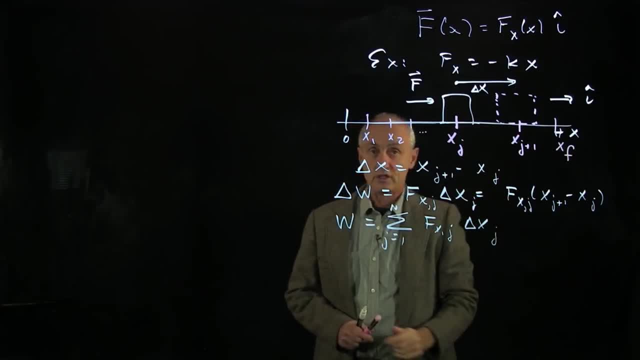 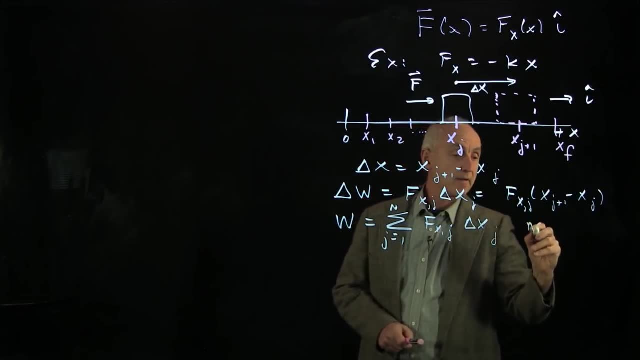 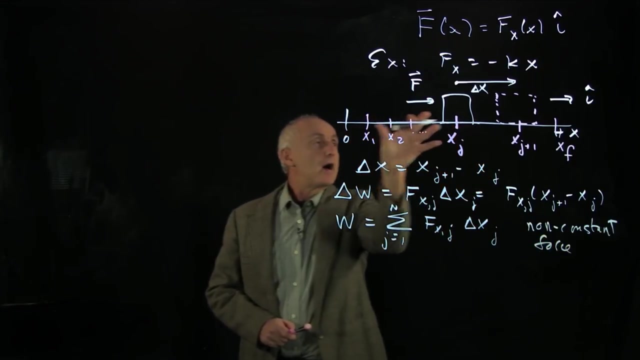 And so this now represents the little bit of work done for all of these displacements, And that is what we define to be the work for a non-constant force. Now, the issue here is about how fine we cut this interval in. 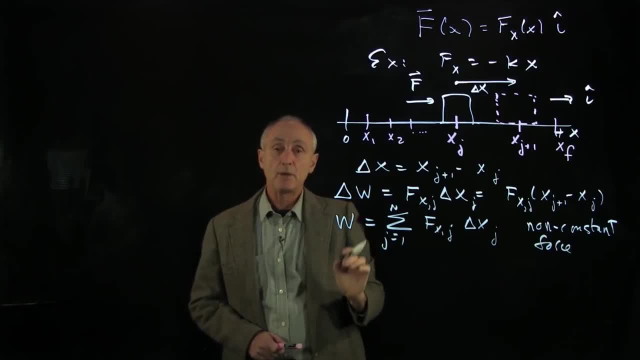 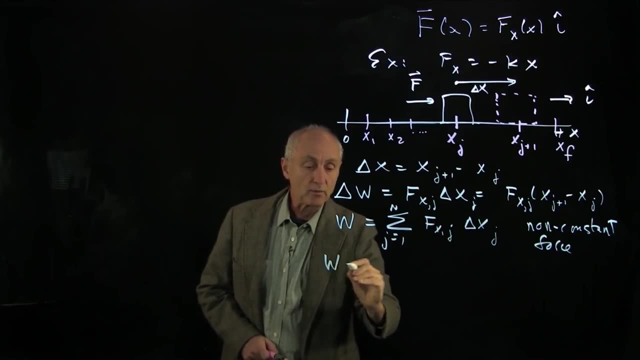 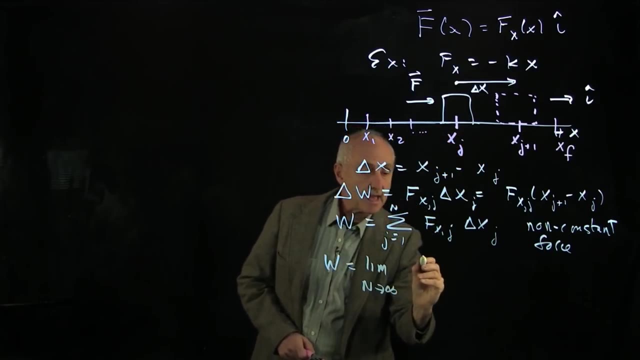 We made n individual pieces, But if we want to ask ourselves what is the limit, as n goes to infinity, then that's what we now need to consider. So what we're doing is we're making smaller and smaller and smaller little displacements. 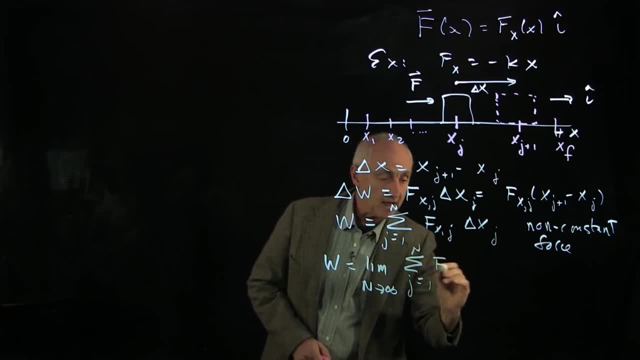 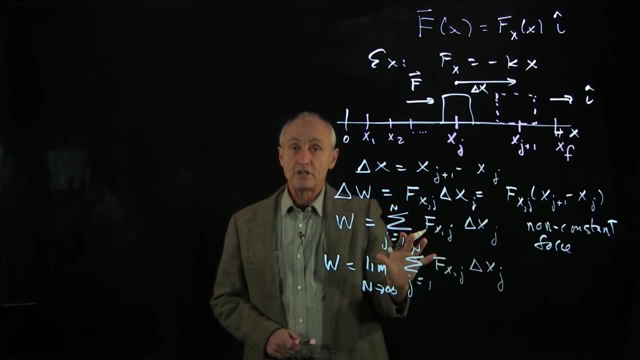 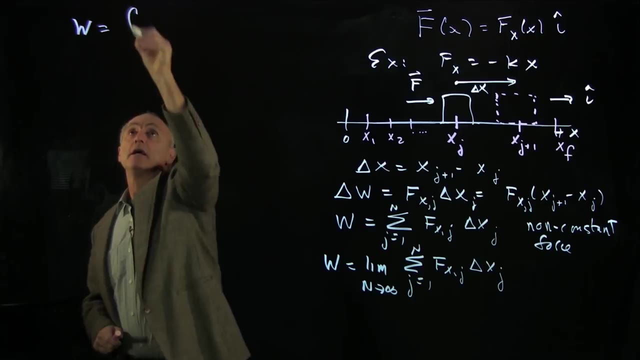 And we're taking this sum, j goes from 1 to n of x of xj times delta xj, And this limit of a sum is, by definition, the integral Of the force with respect to dx. So what we end up with is our work is the integral of f of x. 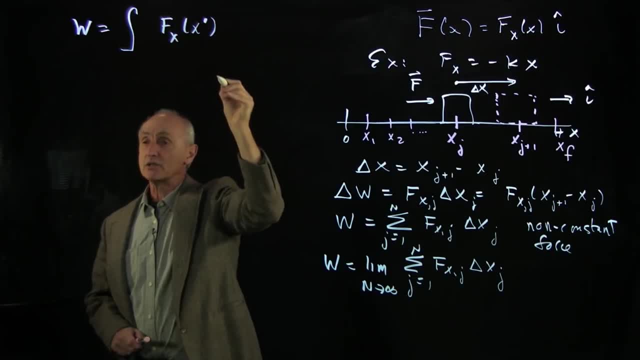 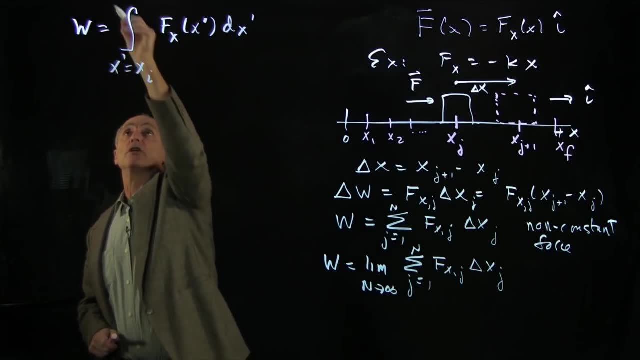 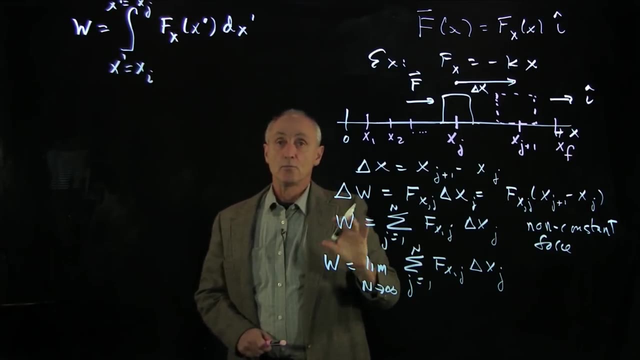 Now it's a function And I'm going to have an integration variable, x prime of dx prime, where x prime is going from our initial position to our final position, And this is now our definition of work, which generalizes a constant force to a non-constant force. 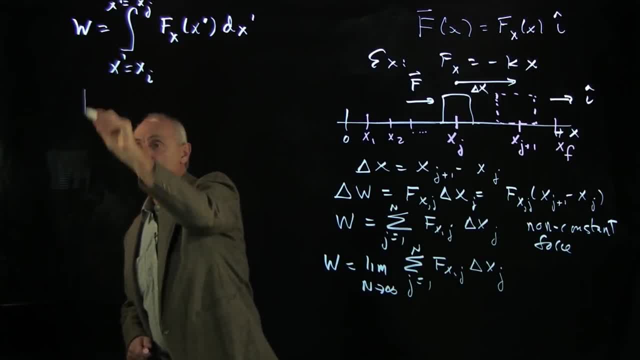 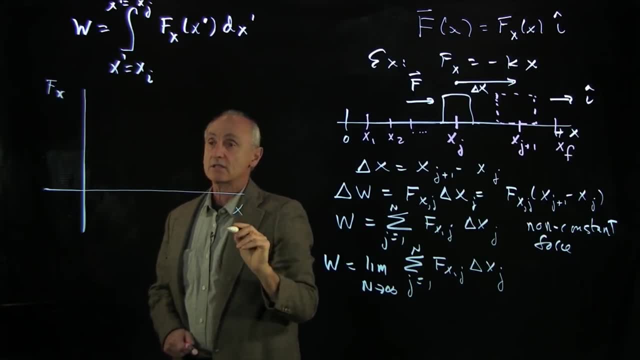 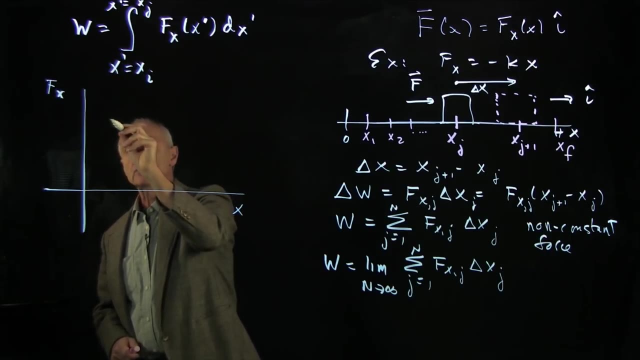 Now again, let's try to look at some type of geometric interpretation. So if we plotted f of x versus x, And now let's consider a case where we have some arbitrary force, So I'm going to just draw the force as if it were arbitrarily increasing. 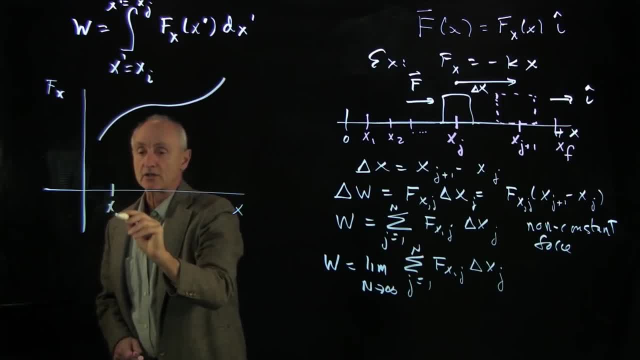 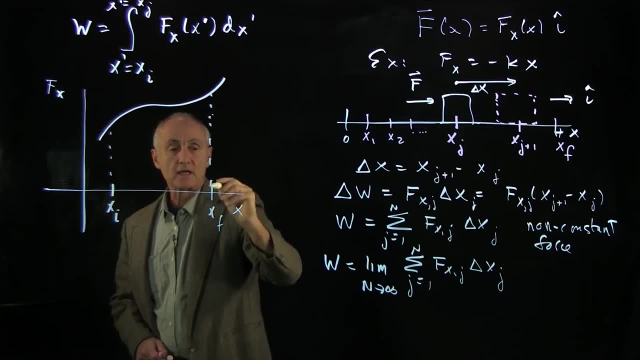 as a function of x. And here's our x initial, And here's our x, And here's our x final. And again we would like to make a geometric interpretation. Let's consider xj, And I'll make this very big xj plus 1, for the sake of visualization. 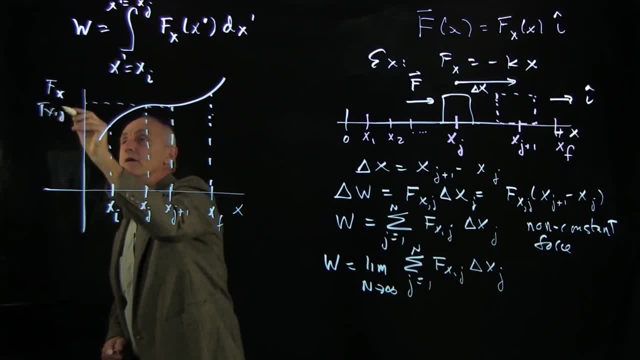 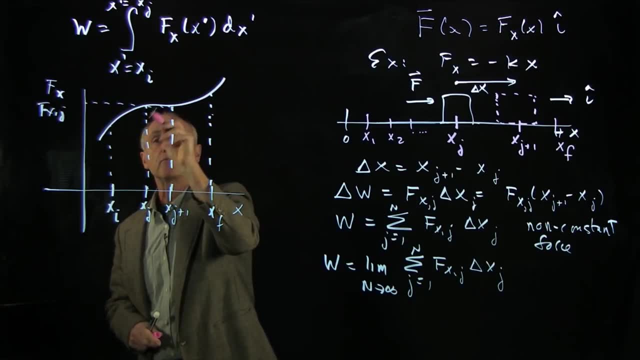 And this value here is f of xj, And so what we see now is that little bit of work like we had for a constant force can be approximated as the area underneath the curve for just this small interval between xj and xj plus 1..